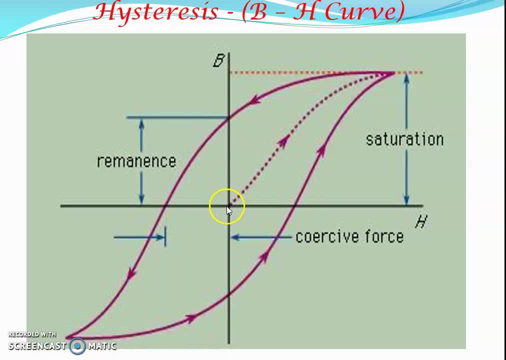 Instead, it has got this much amount of residual magnetic induction, even when the field is reduced to 0. This residual magnetic induction is what is called a remanence, otherwise it is known as retentivity. So in order to bring this residual magnetic induction to 0,, 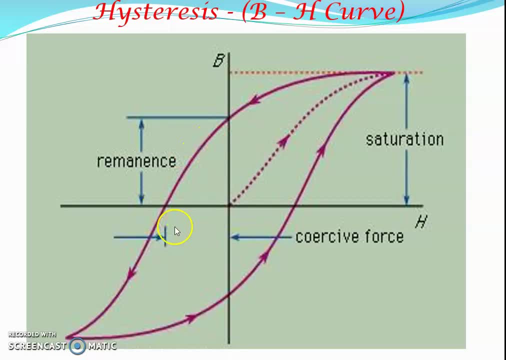 we are going to apply a field in the reverse direction. So when a magnetic field is applied in the reverse direction, at this point the magnetic induction, that is, the residual magnetic induction, comes to 0. So this portion is what is called coercivity or coercive force. 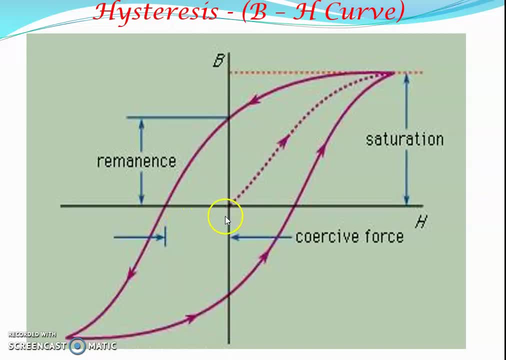 It is the amount of magnetic field that is applied in the reverse direction, in the reverse direction. So this is the amount of magnetic field that is applied in the reverse direction. So this portion is what is called coercivity or coercive force. It is the amount of magnetic field that is applied in the reverse direction, in the reverse direction, in the reverse direction. 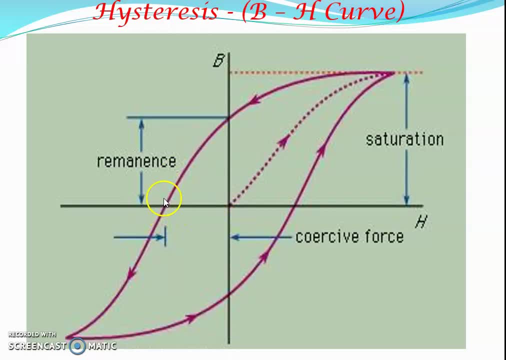 In order to bring this residual magnetic induction to 0.. Now, if we increase the magnetic field in the reverse direction, the magnetic induction takes this shape, and when we decrease the magnetic field, the magnetic induction follows this curve, and we are able to obtain this hysteresis. 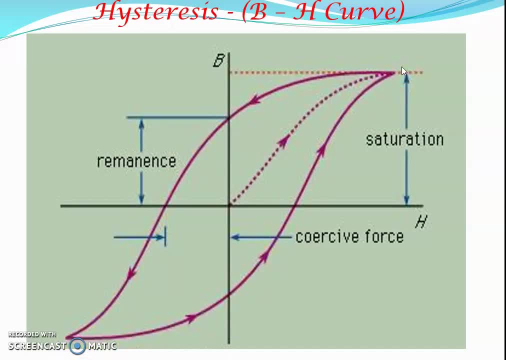 loop when the ferromagnetic material is taken through one cycle of magnetization. Thus, when a ferromagnetic material is taken through one cycle of magnetization, there is a loss of energy in the form of heat, and this loss is what is called hysteresis loss. 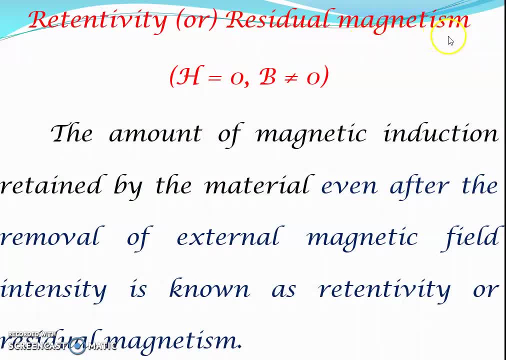 So retentivity is nothing but residual magnetism or residual magnetic induction. That is, even when the applied field is reduced to 0, the magnetic induction is not coming to 0. So that is what is called residual magnetic induction. When magnetic induction is reduced to 0, radish excess will also come back. So there is a loss arrivality called retentivity. 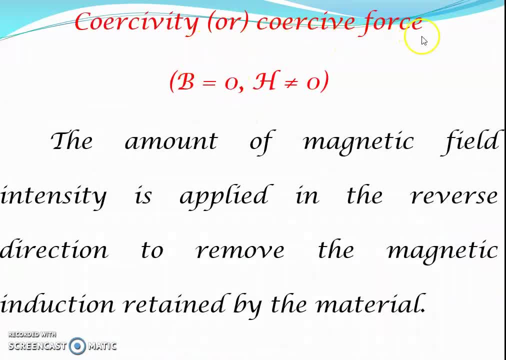 Then coercivity. Coercivity is otherwise known as coercived force. So when the magnetic field is applied in the reverse direction, the magnetic induction is coming to 0. So the amount of magnetic field applied in the reverse direction in order to bring the magnetic induction to 0 is what is called coercivity. So, based upon the 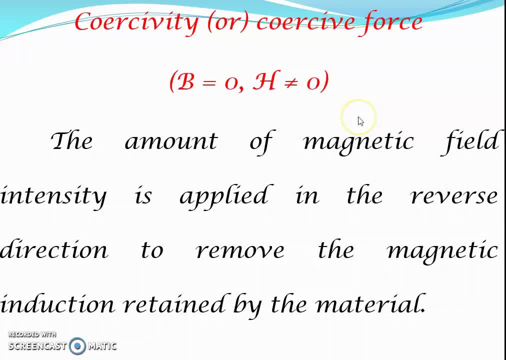 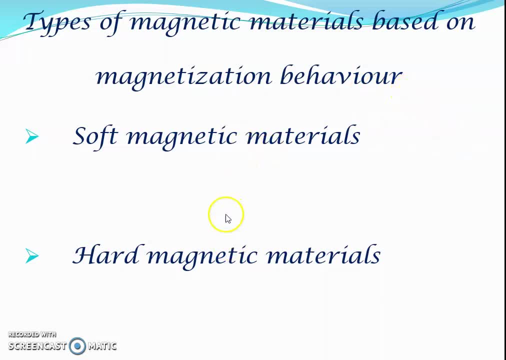 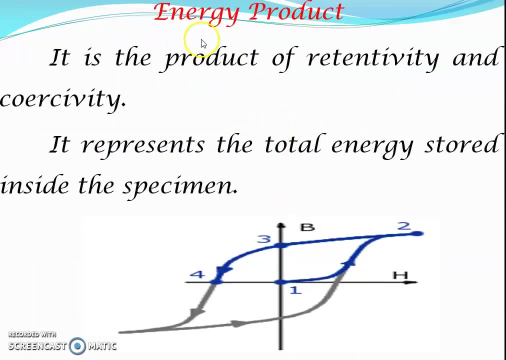 hysteresis lobe, or based upon the magnetization behavior. we have two types of materials: soft magnetic materials, hard magnetic materials. So before that there is a term called energy product. It is the product of retentivity and coercivity. So see the figure In the figure. 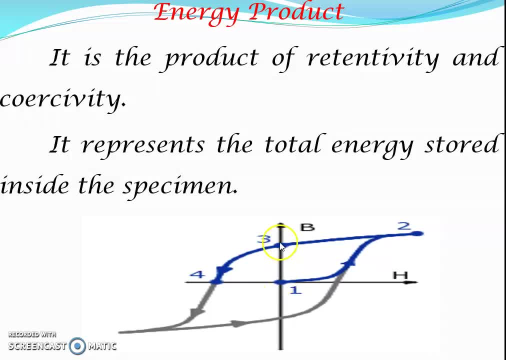 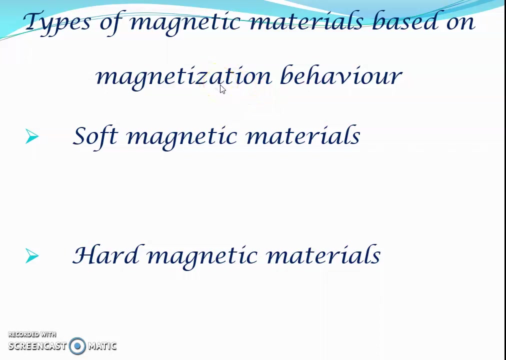 0.13 represents retentivity, the points 1, 4 represents coercivity. So energy product is the product of retentivity and coercivity. It represents the total energy stored inside the specimen. Then, as I told you, based upon the magnetization behavior or based upon the 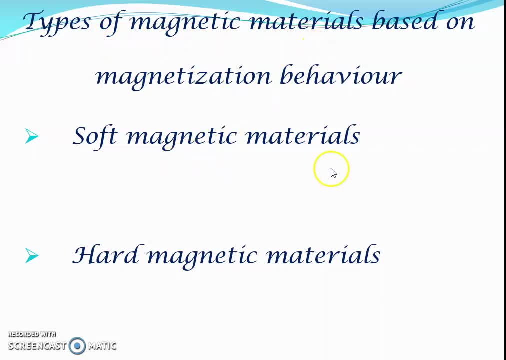 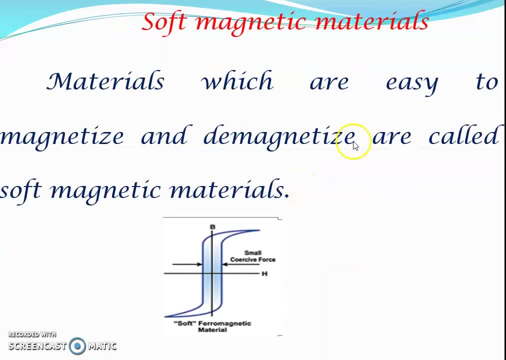 hysteresis lobe. we have two types of magnetic materials: soft magnetic materials. hard magnetic materials- Soft magnetic materials are easy to magnetize and they are easy to demagnetize, That is, they are easily magnetized and also they do not retain their magnetism. 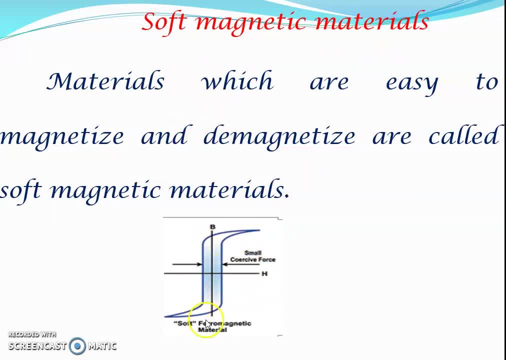 That is what is called soft magnetic materials. So if we see the diagram, the hysteresis lobe area is very small, which means it is able to magnetize easily And it is able to demagnetize easily. So that is what is called soft magnetic materials. 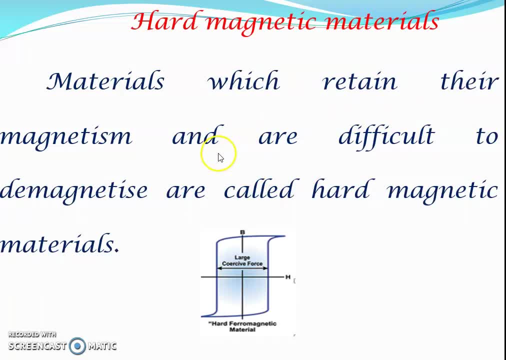 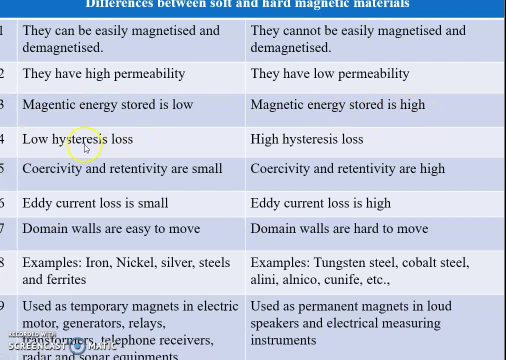 So this type of material is called hard magnetic material. So this type of material is called hard magnetic material. So this type of material is called hard magnetic material. So this type high, Low hysteresis loss. as we saw, the loop area- hysteresis loop area is small in the. 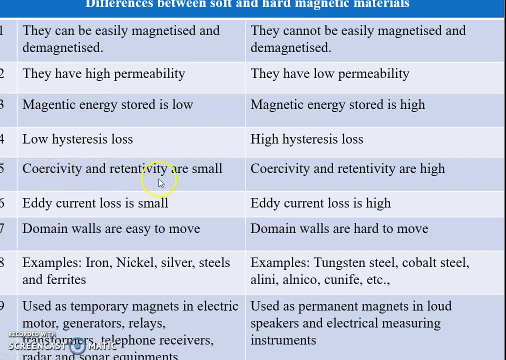 case of soft magnetic materials Also retentivity, coercivity is small. but if we consider hard magnetic materials there is a larger hysteresis loop area, So high hysteresis loss. also retentivity and coercivity are high. Then eddy, current loss is small in the case of soft magnetic. 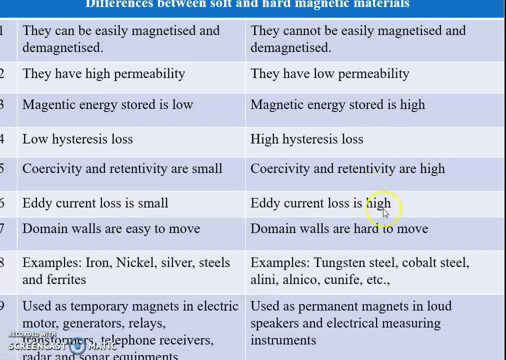 materials, eddy, current loss is high in the case of hard magnetic materials. Here domain walls are easy to move. That is why they are able to easily magnetize and demagnetize. but here domain walls are hard to move, So that is why it is difficult to demagnetize them. 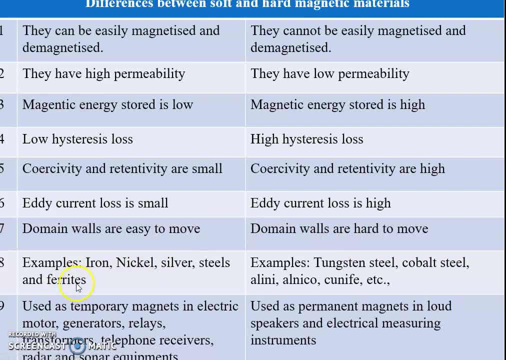 Examples are iron, nickel, silver steels and ferrites. Here examples tungsten steel, cobalt steel, alnico, cuneifel, etc. Soft magnetic materials are used as temporary magnets because they are easily magnetized.